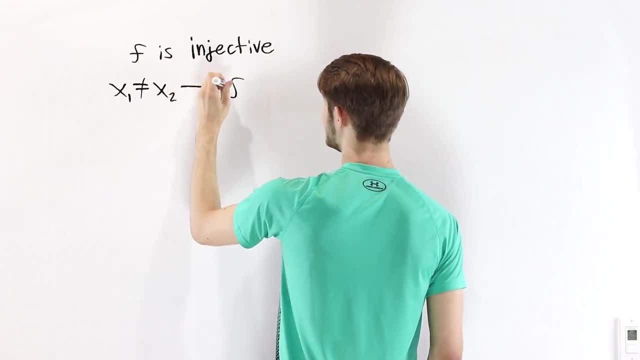 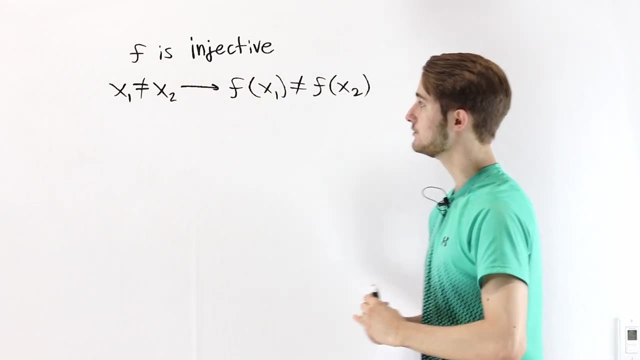 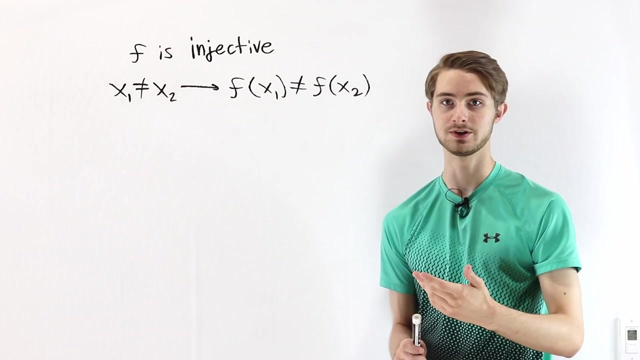 equal to x2,, then it must be the case that f of x1 is not equal to f of x2.. So this is saying that if we have two different inputs that we plug into the function, then we must get two different outputs. Now there's another way that we can frame this statement: using the contrapositive. 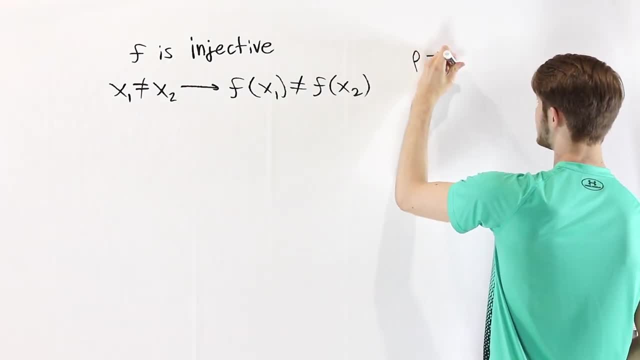 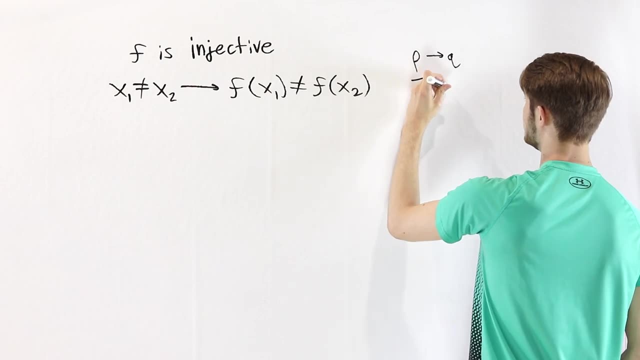 We know that if we're looking at a statement p implies q, like we have here, that's the same thing as its contra positive. So if we're looking at a statement p implies q, like we have here, the contrapositive, which is not q, implies not p. So if we think about how that applies to this, 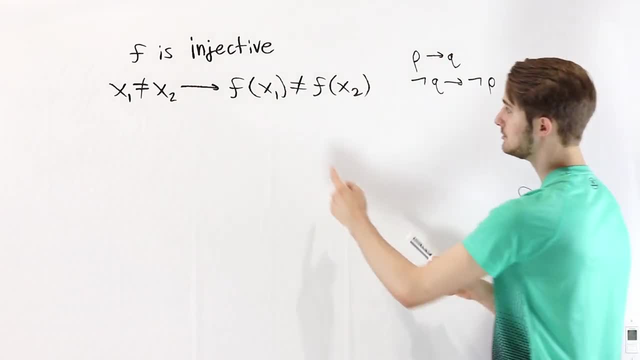 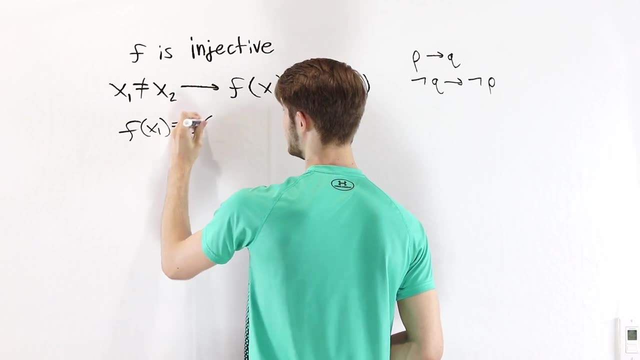 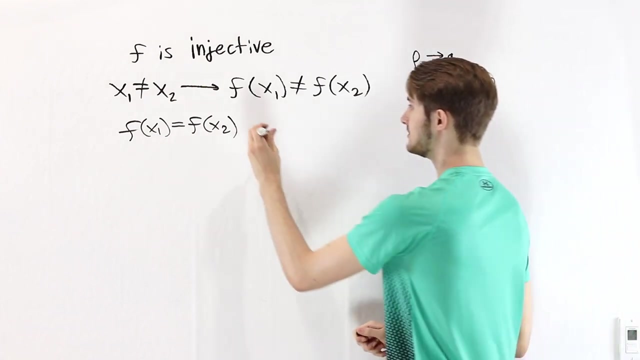 statement here we first want to look at not q. That's going to be the opposite of this second statement. In other words, f of x1 is equal to f of x2.. So this is the negation of our original statement here. We know by the contrapositive that implies not p, which is the negation of this. 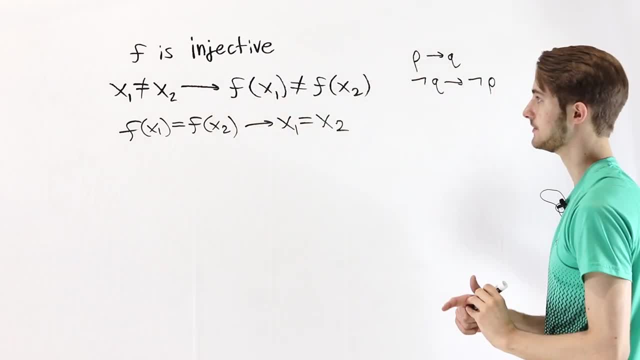 statement here. So if we think about how that applies to this statement here, we first want to look at the contrapositive, which is the negation of our original statement here, And that would be: x1 equals x2.. So this is saying. another definition of injective is that if we get the same output to 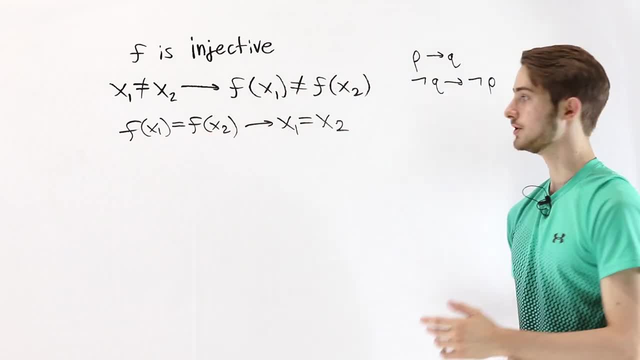 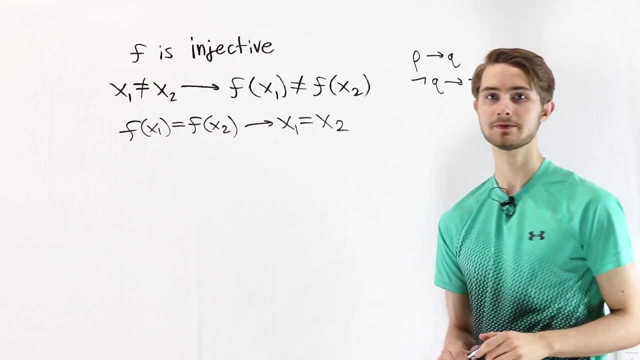 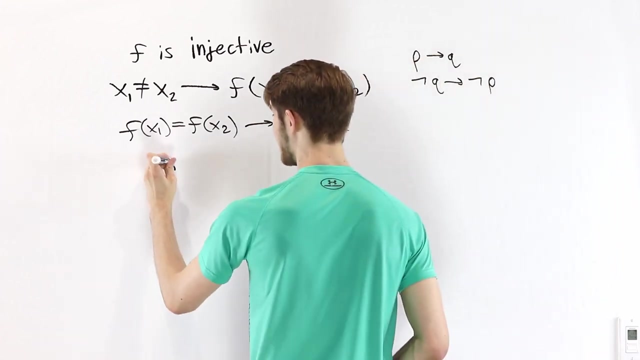 our function for two inputs, then those inputs must have been the same. Every output has at most one input, And that also has an important consequence when we look at multiple different inputs. So let's say we have an input space for our function and we're looking at a function. 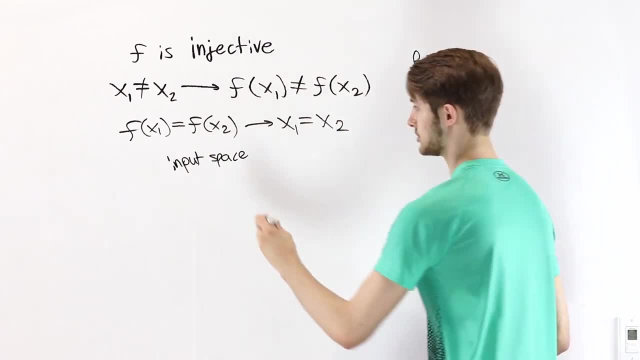 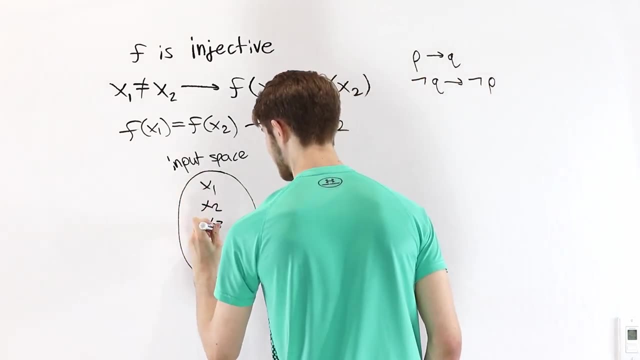 that we can input into our function, Some set of values that we can input into the function. That would also be called the function's domain. So we have x1,, x2, x3, and so on to let's say, xn. So 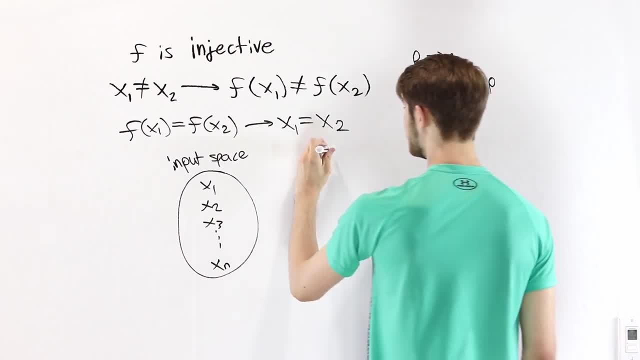 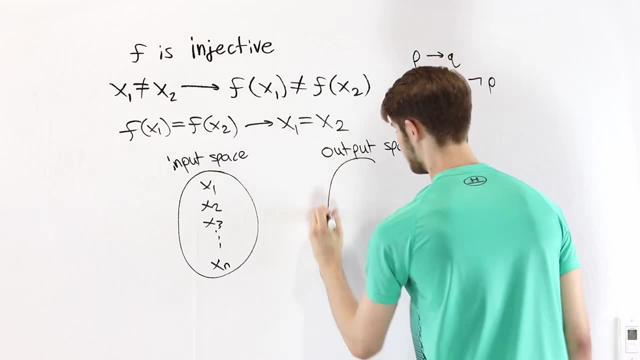 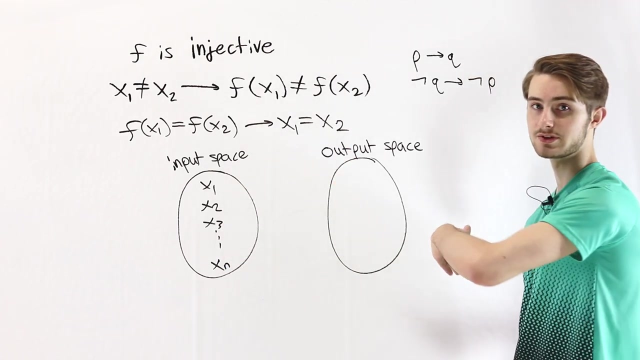 these are inputs that we can give into our function. Over here we have the output space, which is also called the codomain of our function. So this output space contains all of the values that we could get if we input something into the function. So this could be y1,, y2,, y3, all the way.